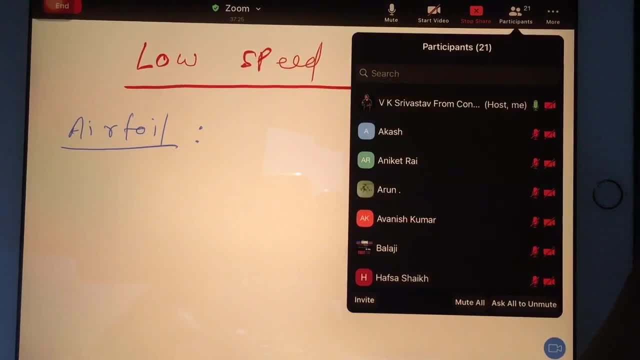 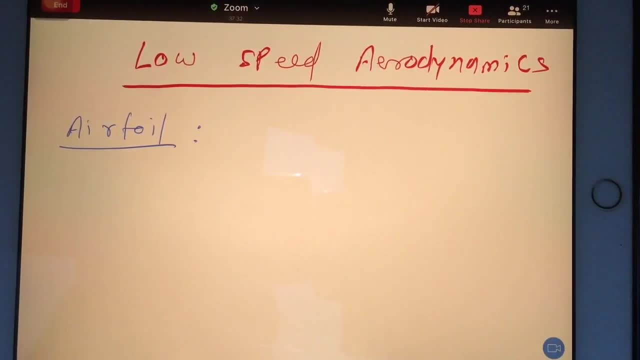 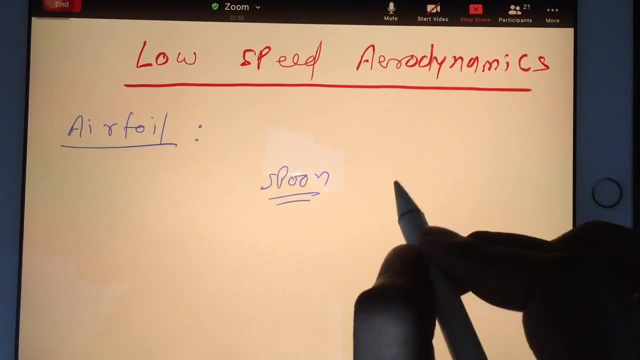 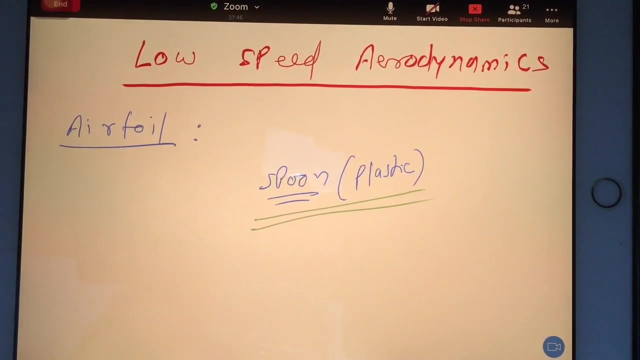 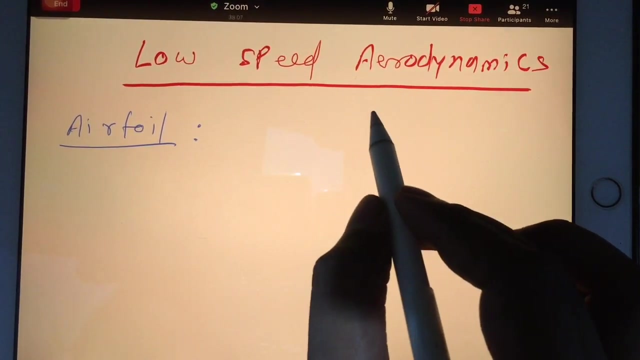 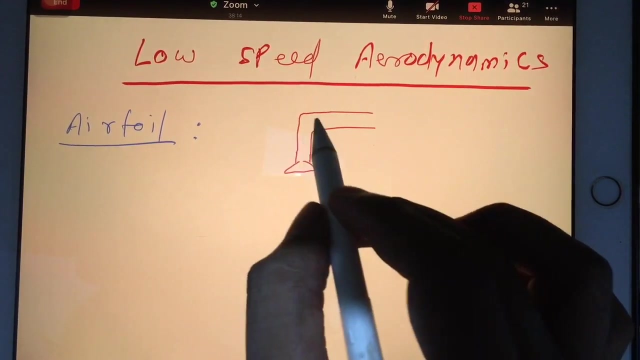 In your low speed aerodynamics you will perform one experiment. Because we are not in live class otherwise I could have done the performance. So you will do one thing. You need a spoon. Actually you need a spoon. That spoon you can get from but must be plastic. It must be plastic spoon. So your experiment will go well. But if you don't have plastic spoon you can try with your steel spoon. Because steel or some metal spoon is easily available in home. But actually with that spoon the process will not work properly. And it is my own experience. That's why I am giving you this. You see. What will you do? You take one spoon. See you do one thing. You have tap water right? Tap water in your home. Tap water in your bathroom or basin or somewhere. Tap water. So open the tap water with full speed. With very high speed you open the tap water. 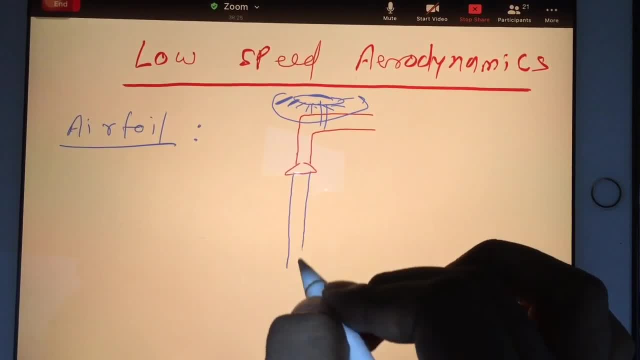 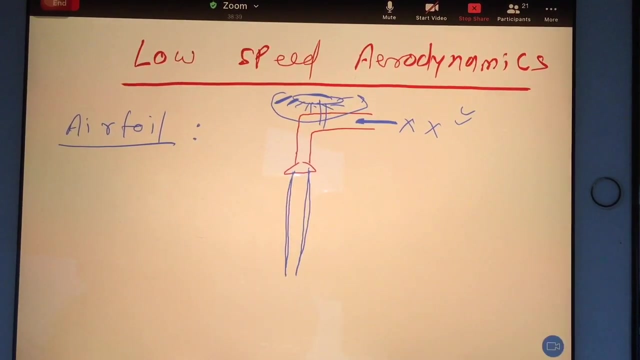 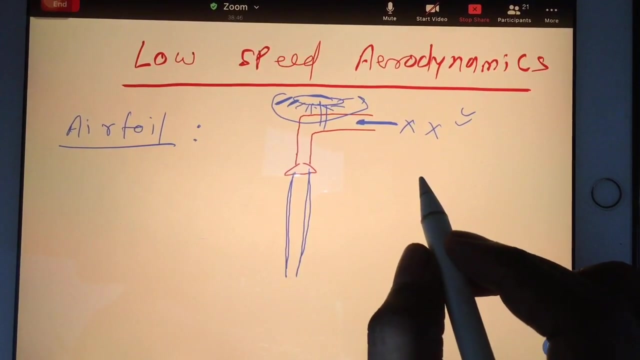 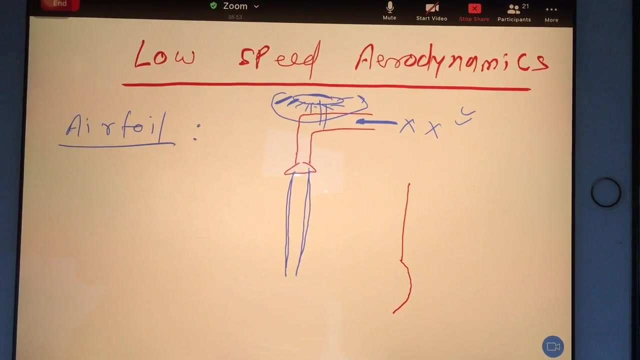 Okay. So the tap water will be coming down. And make sure it should not come as turbulent. Little bit turbulent is okay. It should come as laminar. Okay. Even though turbulent is coming this experiment will work. Okay. Now you do one thing. You take the spoon. Okay. I am drawing the lateral view. So my spoon will look like this. This is the handle. And the lateral view I am drawing. drawing lateral view okay this is the lateral view so you put your spoon in the flow you put your spoon in the flow then you know what will happen the moment you will put the spoon in the flow a spoon will tilt this side automatically so tonight after lecture or tomorrow you can perform 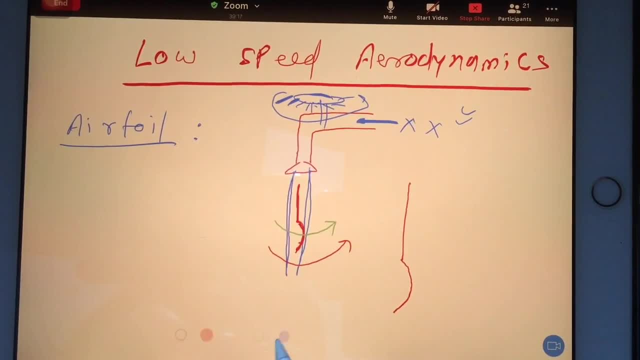 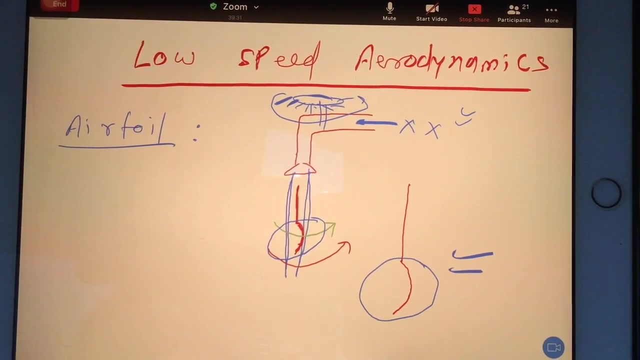 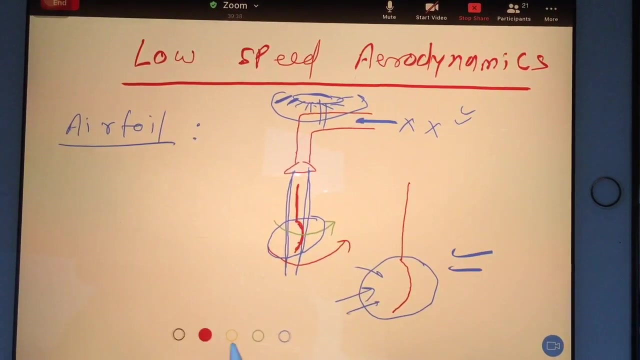 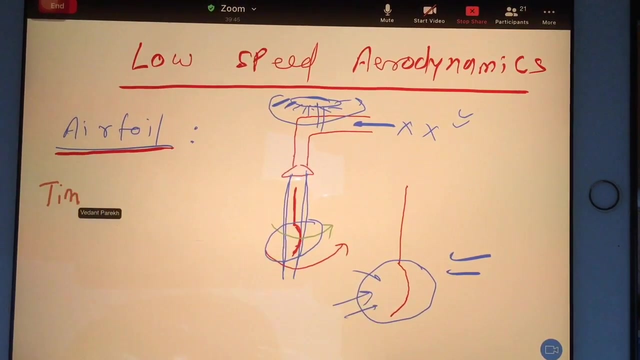 this why it is happening because of this curvature because of this guy okay and whoever is watching this concept on YouTube they will they will be amazed after knowing this yes it is very simple you can you can perform at home right guys everyone you will be like amazed yeah this is happening it is very easy so actually what is airfoil yeah time is about to over